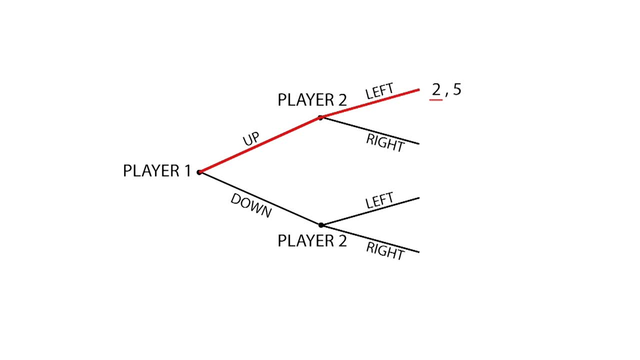 the combination up-left will have a payoff of 2 for player 1 and a payoff of 5 for player 2.. Let's say the final payoffs for each outcome are as follows: It is important to remember that the first payoff corresponds to player 1 and the second 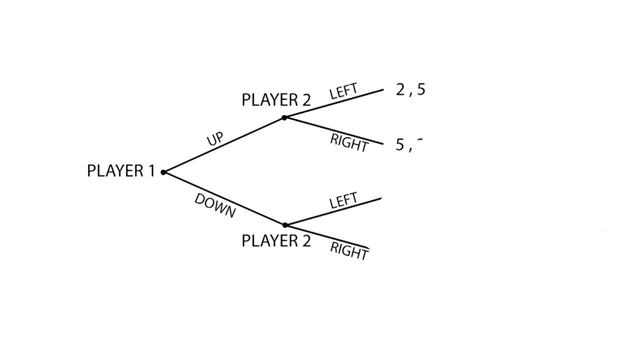 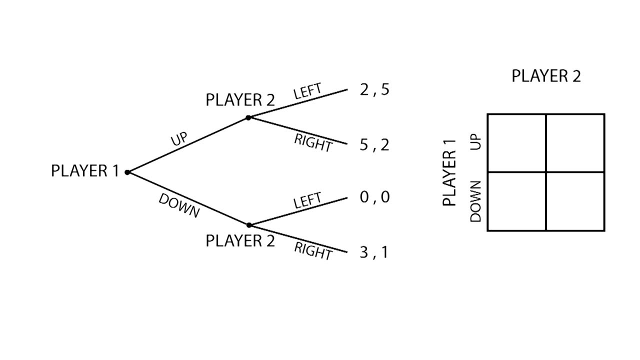 to player 2.. We can also represent the game using the strategic form. Rows represent player 1's strategies up and down, while columns correspond to player 2's strategies right and left. If player 1 goes up and player 2 goes right, Final Payoffs- Equal- are 5, 2.. 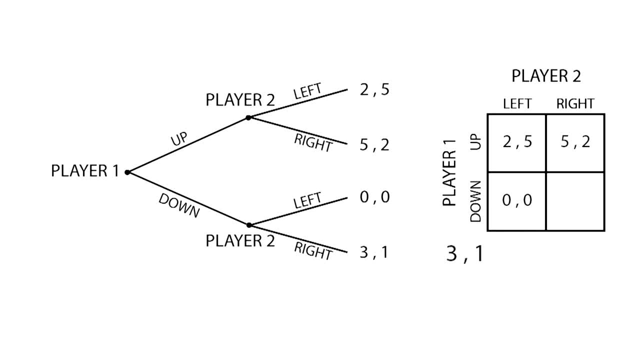 Using this same procedure, we are able to fill out the entire matrix. Here's how we would do it. We can also change the column from column B to column C to column B. If we change the matrix, Let's look for the Nash equilibrium of this game. Player 1 knows that player 2 will. 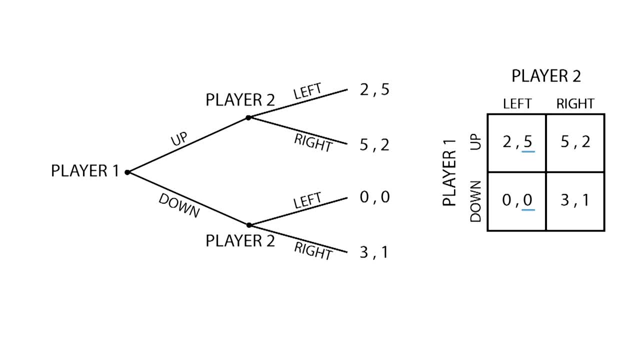 rather go left, since his expected payoff would be greater. Therefore, player 1 chooses to go up, since this will derive in a higher payoff. Player 2 knows that player 1 will rather go up, since his expected payoff would be greater. Therefore, player 2 chooses to go left. 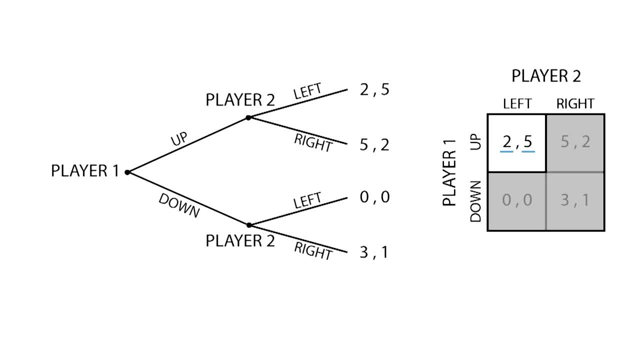 since this will derive in a higher payoff. Therefore, we find that up left is a Nash equilibrium, since going up is the best strategy player 1 can choose and going left is the best strategy for player 2, considering the other player's strategy. However, since this is a 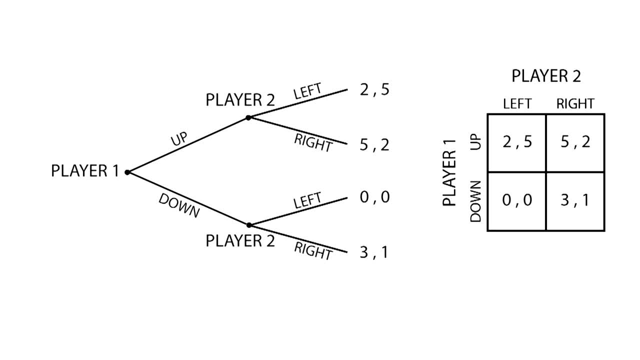 sequential game. this is not a perfect equilibrium. In order to find the sub-game perfect equilibrium, we must do a backwards induction, starting at the last move of the game, then proceed to the second to last move of the game and then proceed to the second to last move of the game. 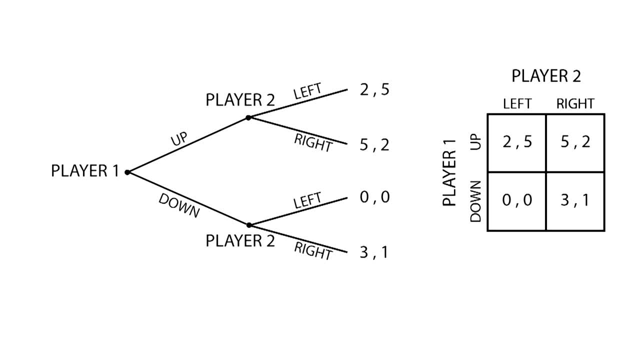 In this particular case, we know that player 2 will choose left if player 1 goes up and right if player 1 goes down, since these are the moves that maximize player 2's payoff, Because there is complete information and therefore each player's payoffs are known. 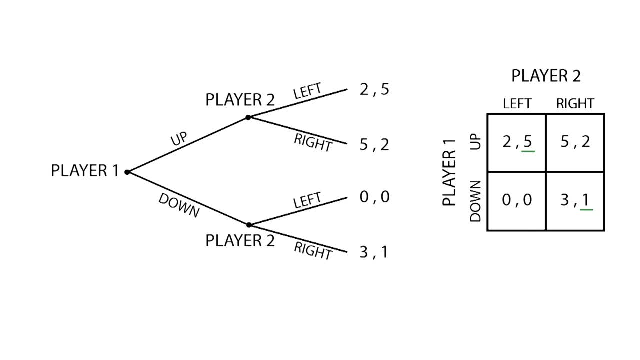 player 1 knows these choices in advance and will therefore choose to go down because his final payoff will be greater. Therefore, down right is the perfect sub-game equilibrium. Sub-games are of special importance when analyzing repeated games, also known as supergames, since repetition is easier to analyze using a game tree with multiple. branches.